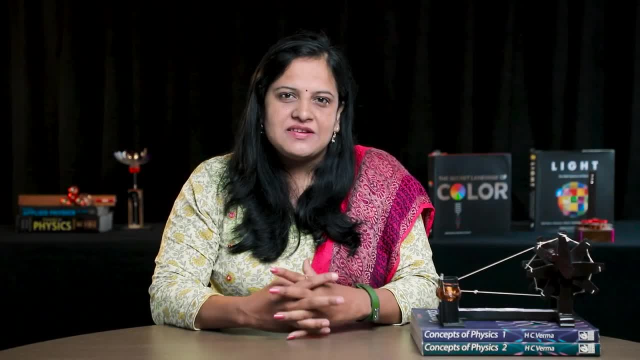 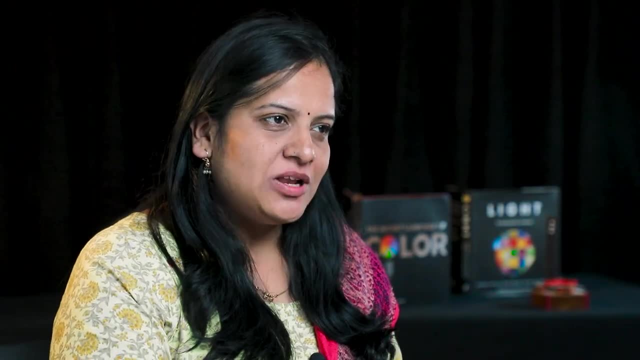 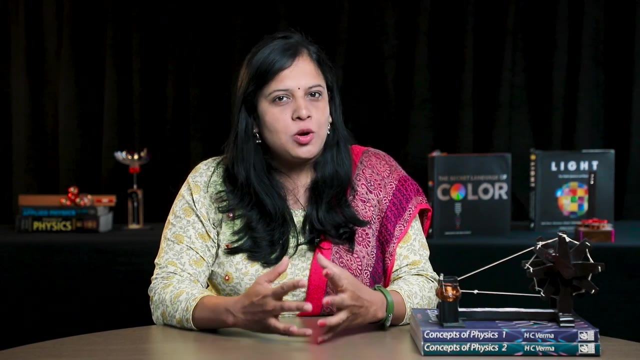 Activity Centre at ISA Pune. She has also tried this lesson with her students and she has shared her experiences with us. So welcome to this physics video lesson plan on an very interesting topic that is, electricity and magnetism and their relationship. Students normally learn this concepts in their 8th and 10th grade. We have tried to make this. 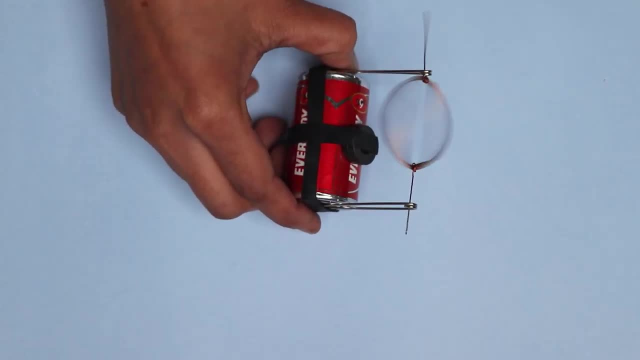 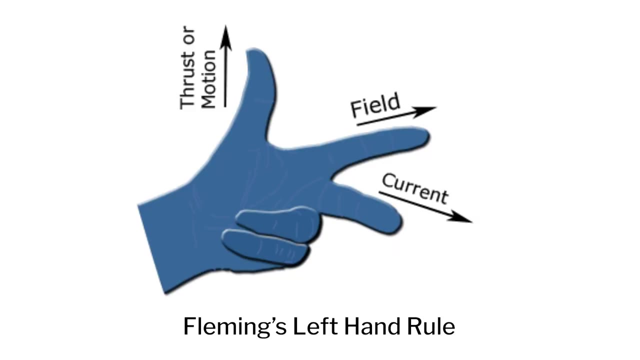 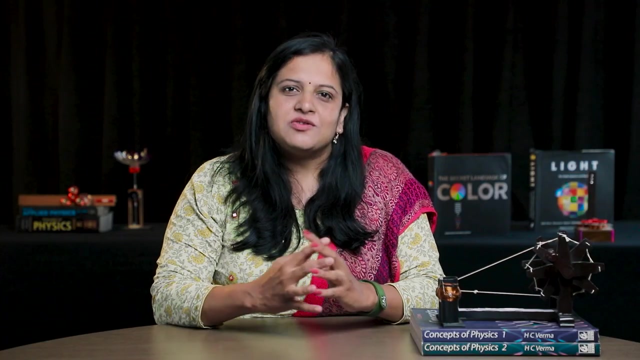 lesson more interactive and activity based. We will see how to make a DC motor. Faraday's Electromagnetic Induction, Fleming's Left Hand and Right Hand Rule, Effects of Eddy Current. So let's start with a very interesting activity to see the relationship between electricity. 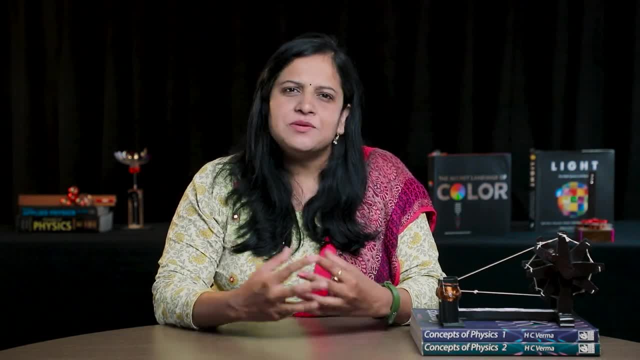 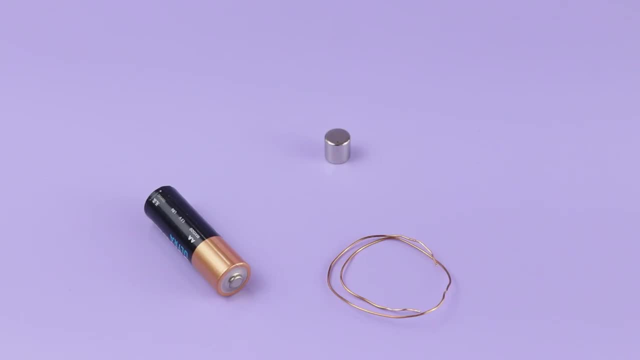 and magnetism in action, And for that we have a simple toy called as valve motor. Let's see how to make it. To make a valve motor we need neodymium magnets, a bare copper wire and a 1.5 volt battery. Twist and wrap pieces of bare copper wire into different shapes. 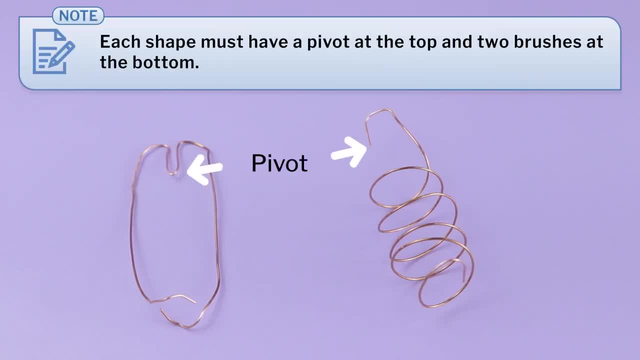 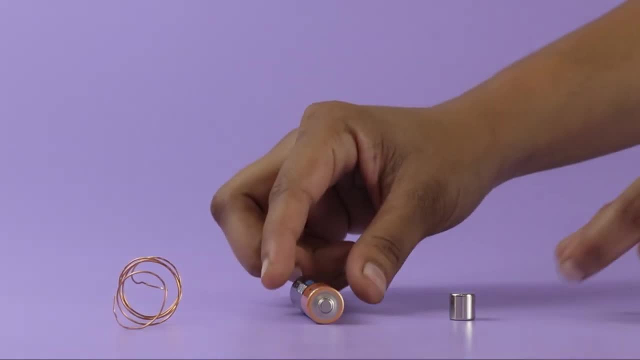 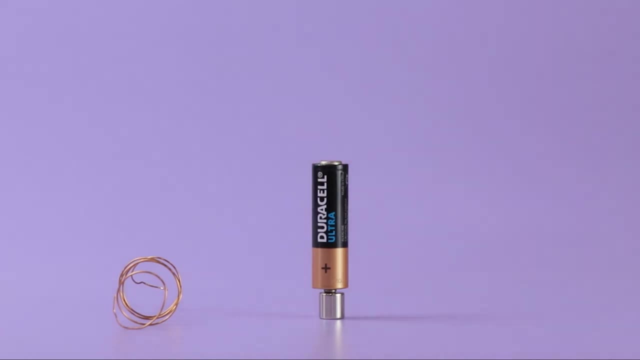 with only two conditions: Each shape must have a pivot at the top and two brushes at the bottom. Bring a 1.5 volt battery near a strong neodymium magnet. Place the battery on the magnet. Balance the pivot of your copper coil on top of the battery and bring the battery. 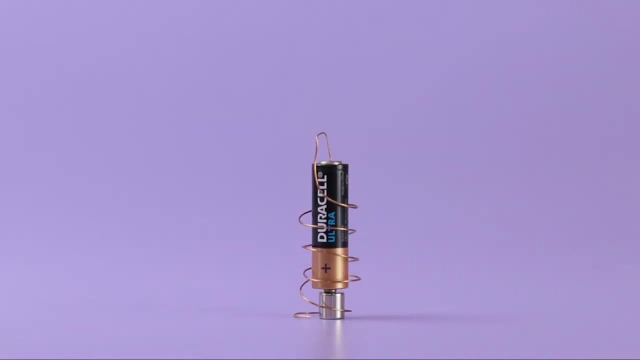 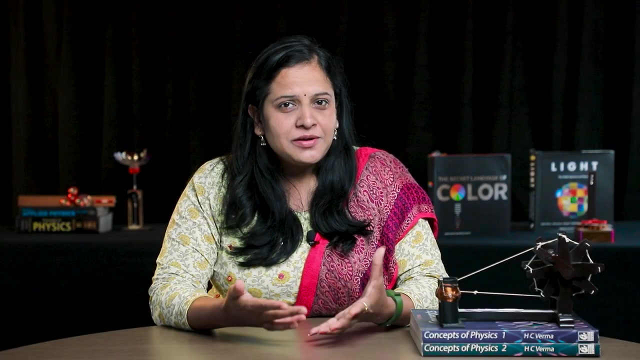 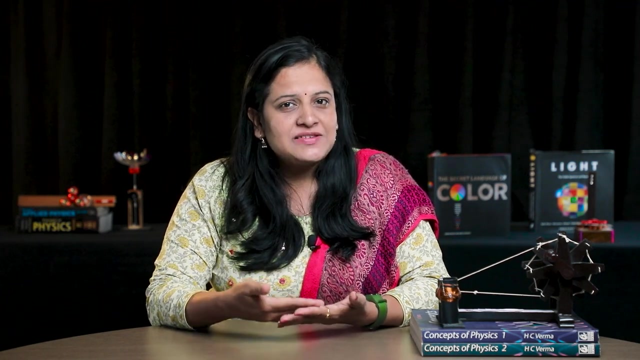 in contact with the neodymium magnet. Wow, the coil starts spinning, Isn't it interesting? So here, if you remove the contact between the brushes and the magnet, the coil does not move. Also, if you place an insulating material between the battery and the pivot, 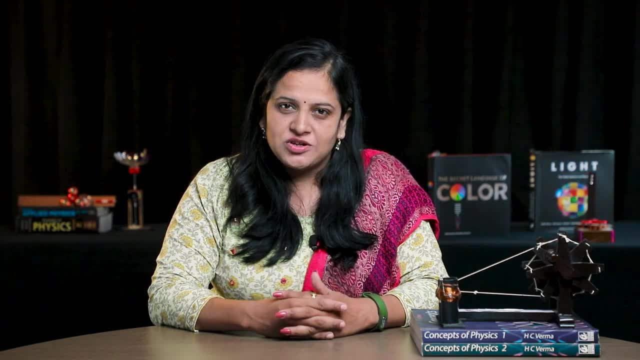 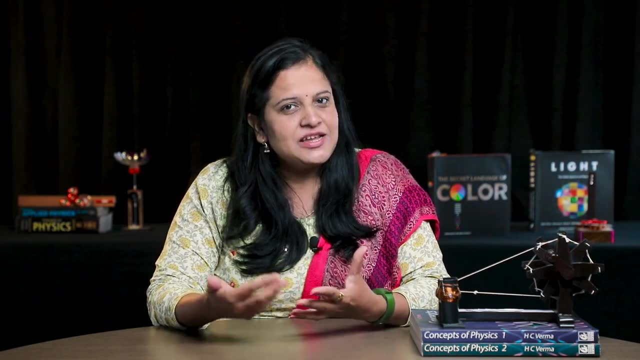 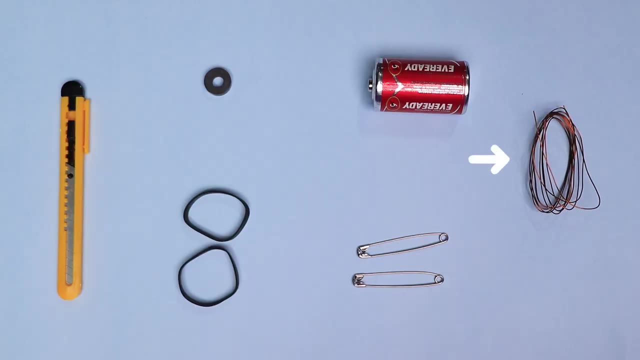 then also, the coil is not going to move. You can ask this question to the students, that why does this happen? So let's see one more interesting activity. For this we need a copper coil, a battery, two magnets, two thin ring cutouts from a rubber tube and two safety pins. Wind 10. 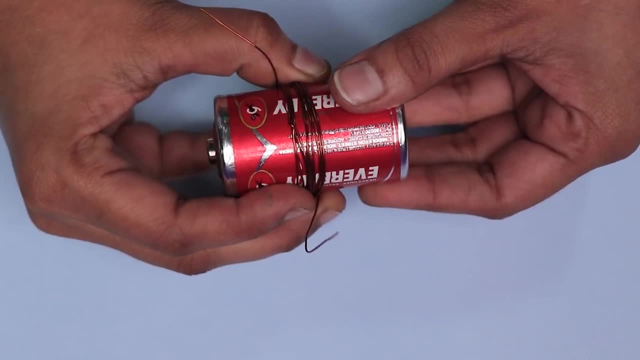 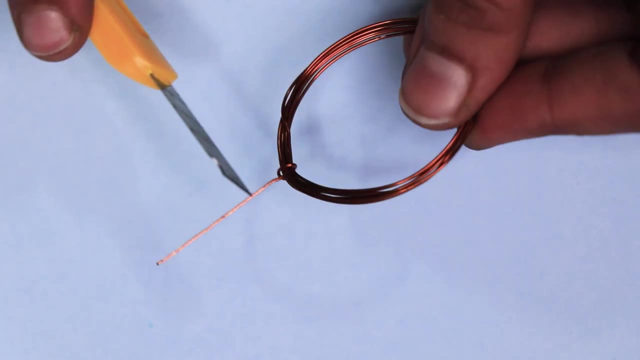 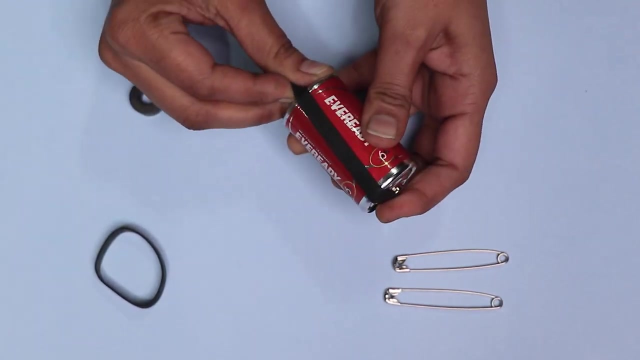 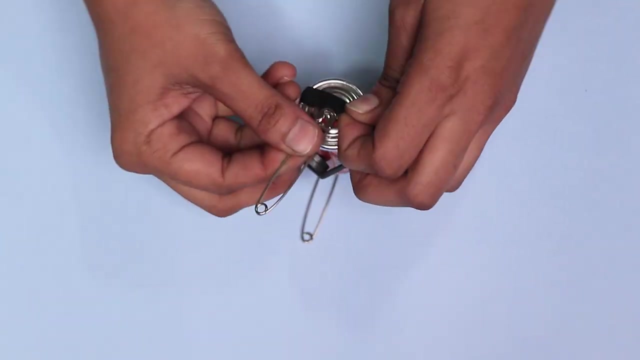 turns of 20-gauge insulated copper wire around a battery. Keep the two ends open and diametrically opposite. Remove the insulation completely. Use the rubber rings to hold everything in position. Attach two magnets and safety pins to the battery as shown here. Insert two ends of the coil through the holes of the safety. 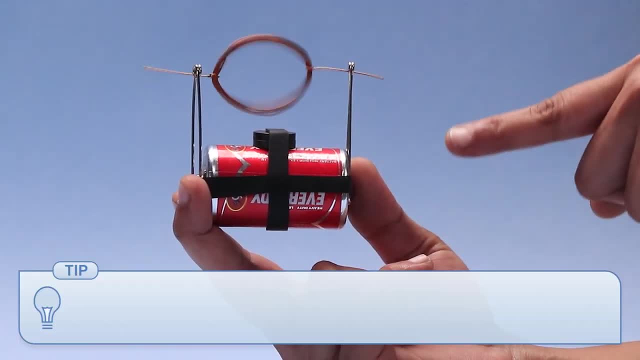 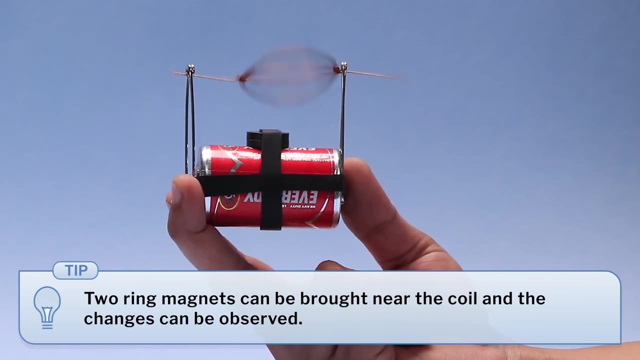 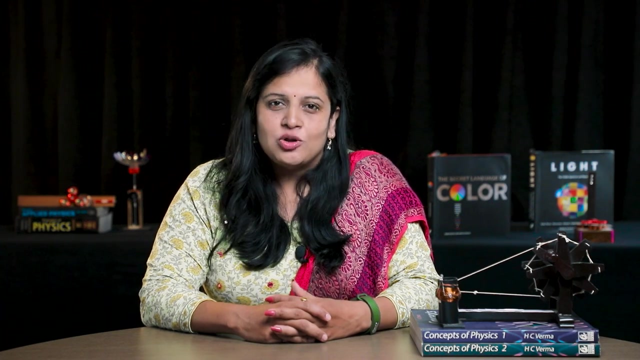 pins. Give a slight push to the coil, It starts spinning. This is a demonstration of Fleming's left-hand rule: How to use a safety pin. To remember Fleming's left-hand rule, we take help of a very popular mnemonic FBI. 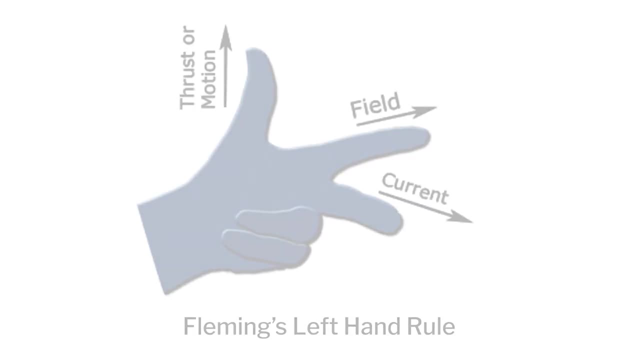 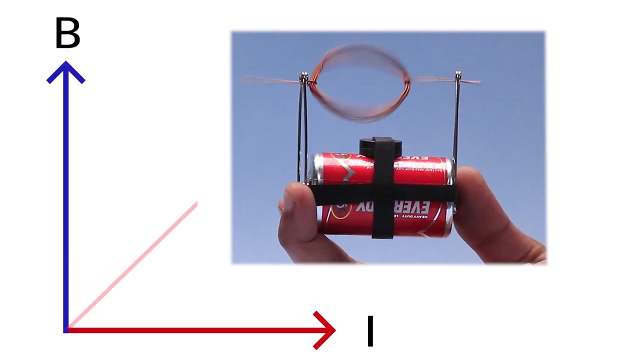 Though it might seem like CID, but over here in FBI, F stands for force, B stands for magnetic field and I stands for. current Fleming's left-hand rule states that when a current-carrying conductor is placed in external magnetic field, then the conductor 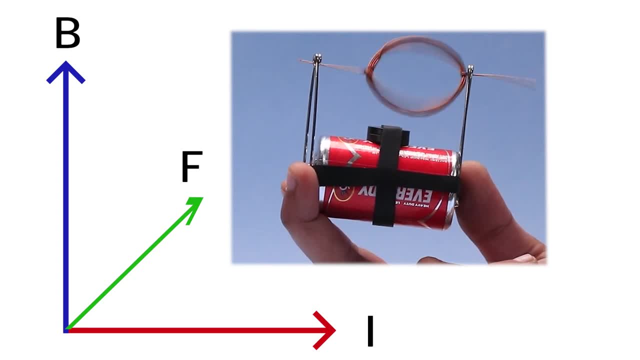 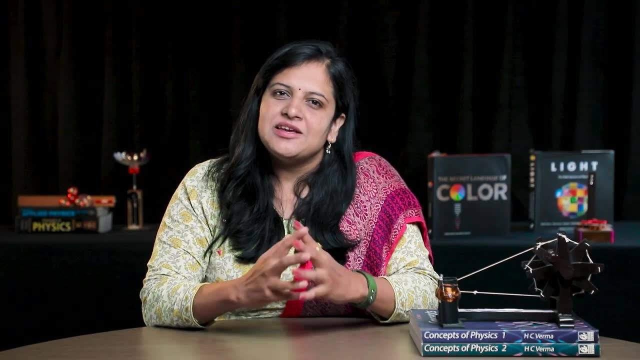 experiences force. This force is perpendicular to the direction of the magnetic field. The force is perpendicular to the direction of the magnetic field. This force is perpendicular to the magnetic field and it is also perpendicular to the direction of the current. So let's see Fleming's left-hand rule over here. I have my left hand and these three. 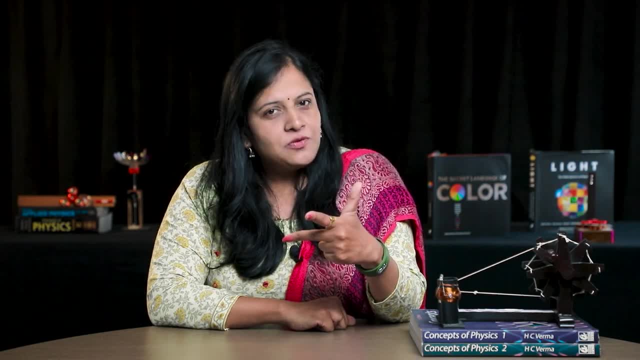 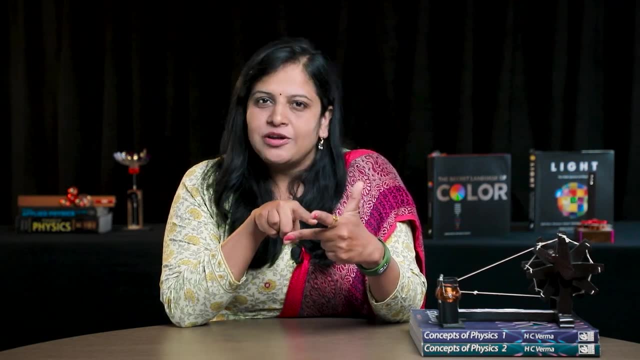 fingers are perpendicular to each other, So, according to Fleming's left-hand rule, the forefinger denotes the direction of the magnetic field, the center finger denotes the direction of the current and the thumb denotes the direction of the force created. So perhaps, 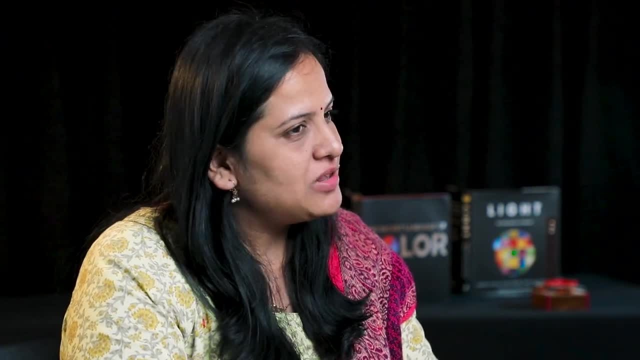 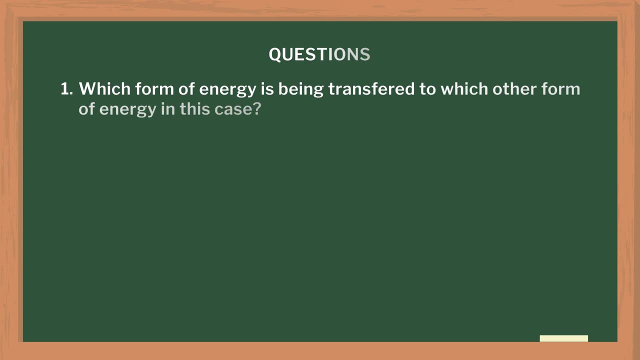 during the demonstration. you can ask students to use a safety pin. You can ask students to find out these directions. You can also ask them the following questions: To which form of energy is getting transferred? to which other form of energy here? Will the coil rotate if you take away the magnets? 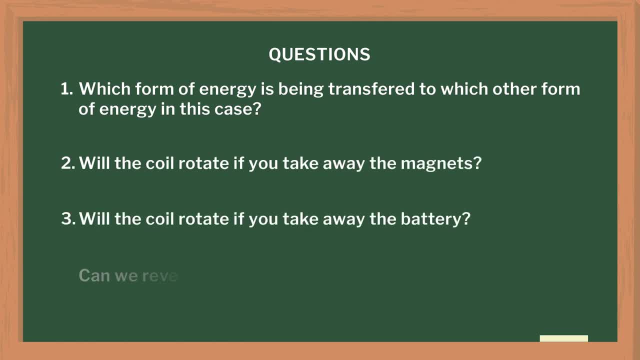 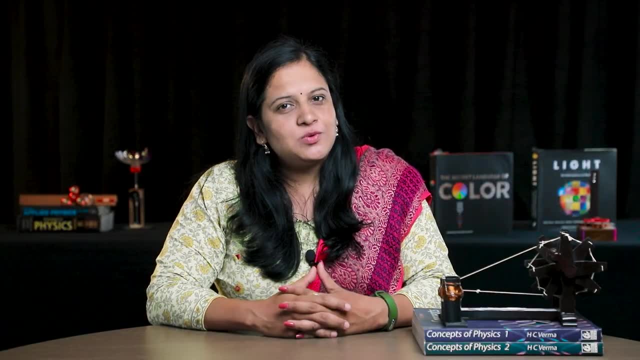 Will the coil rotate if you take away the battery? Can we reverse the direction of rotation of the coil? If yes, then how? You can ask these questions to the students and have an interesting discussion on this. This brings us to the end of this video. Thank you for. 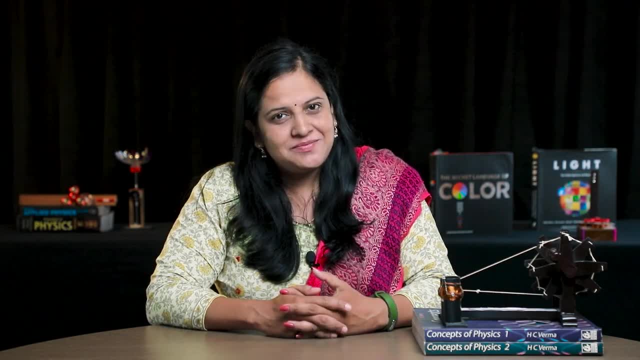 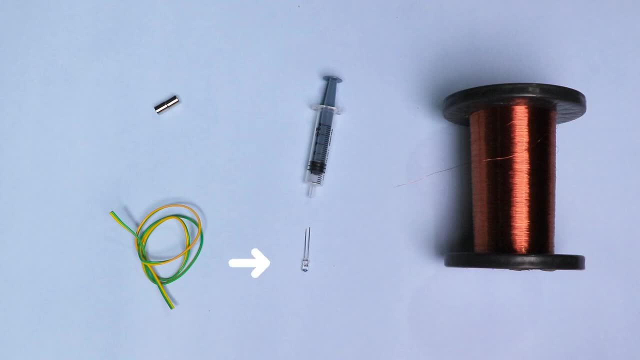 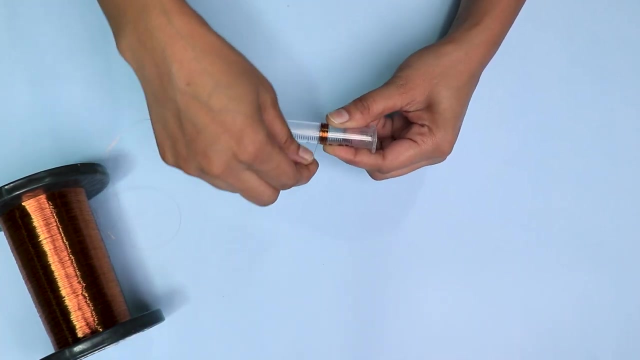 watching For this activity. we need a 5 mL syringe and LED, that is the light-emitting diode. few neodymium magnets that can fit loosely inside the syringe. a coil of copper wire. remove the rubber cap from the piston of the syringe. wind copper wire around. 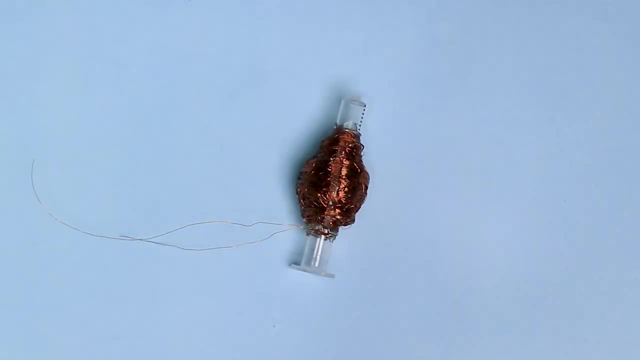 the middle of the syringe thousand times and cut the coil Carefully. strip away the insulated wire and remove the rubber cap from the piston of the syringe. Wind the copper wire around the middle of the syringe a thousand times and cut the coil Carefully. strip away the 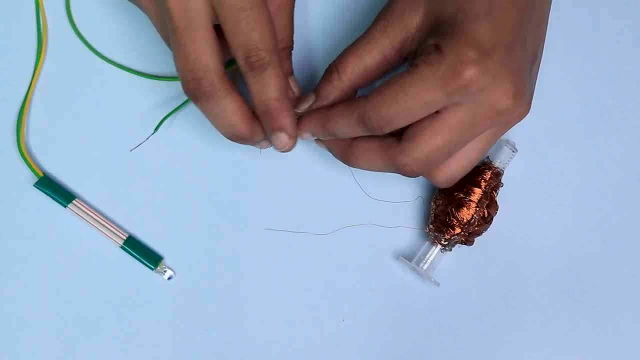 rubber cap from the piston of the syringe. wind copper wire around the middle of the syringe and remove the rubber cap from the piston of the syringe. Attach the two ends of the copper coil to the two terminals of the LED. Insert the neodymium. 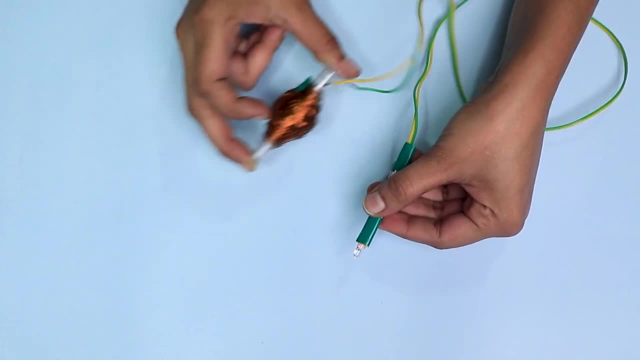 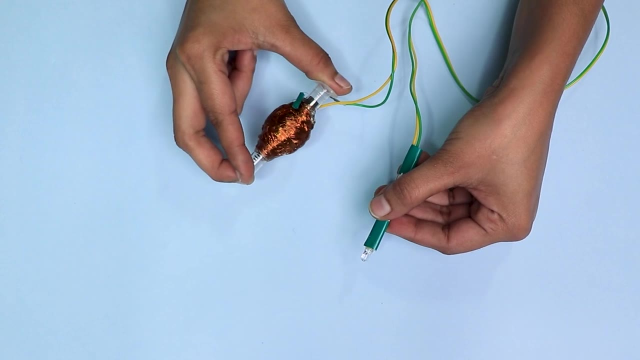 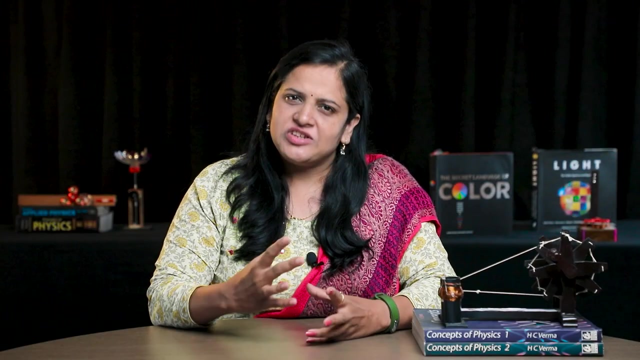 magnet into the syringe Vigorously. shake the syringe lengthways to light up the LED. Let's slow it down a bit. Did you notice a change Now? let's shake it faster. The bulb got brighter right. So here, if we shake the syringe more vigorously, the bulb would revealed so we could shake. 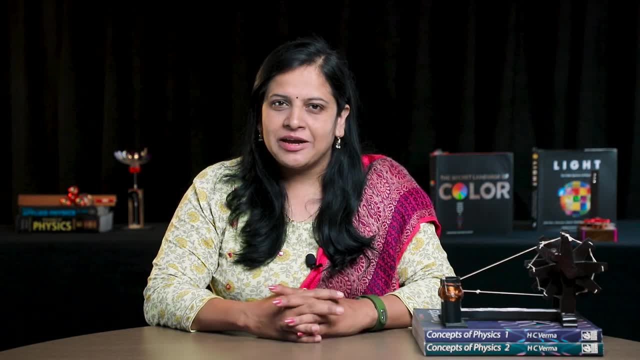 the syringe more vigorously, The bulb could walk to the next site. All right. now see, the change is coming. this time the bulb got brighter still. the bulb got even brighter. the speed of the magnets is increased. that means the current is increased. the direction of the 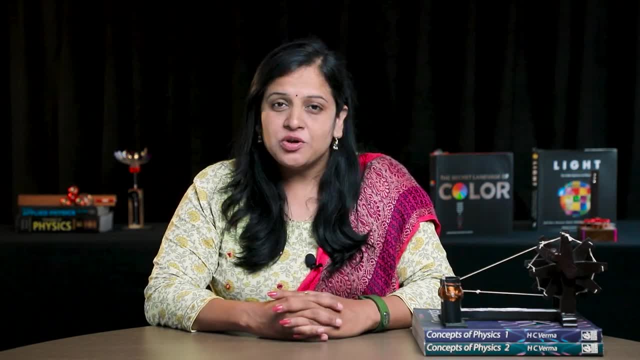 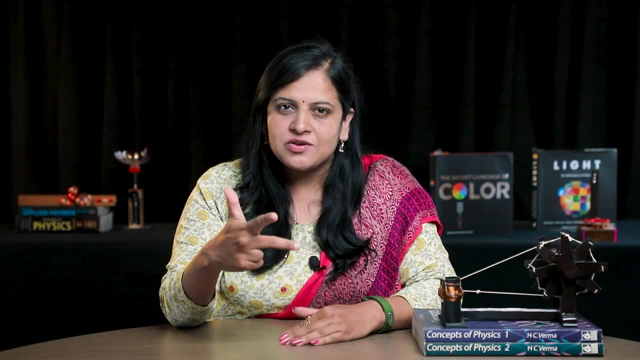 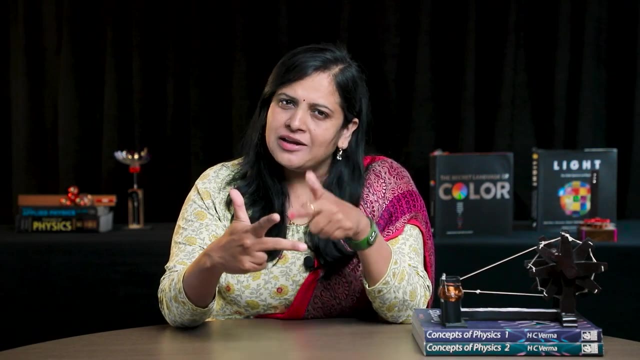 current depends on the direction of the magnetic field. so here again we take help of our old friend fleming and his right hand rule. if i hold my right hand and the fingers of the right hand perpendicular to each other, that means the middle finger, the forefinger and the thumb are exactly. 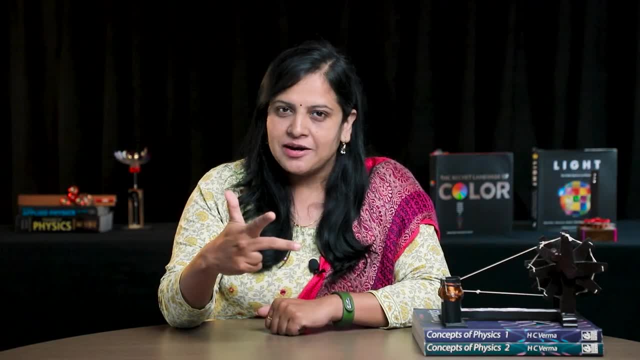 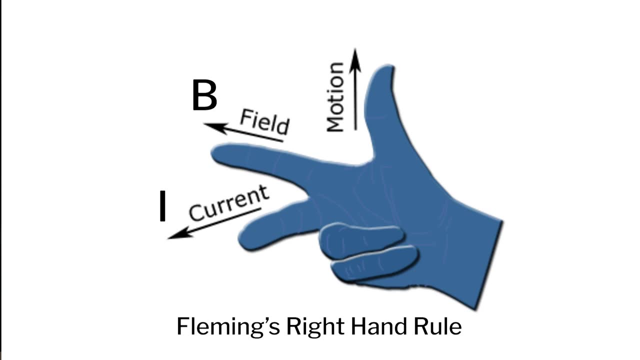 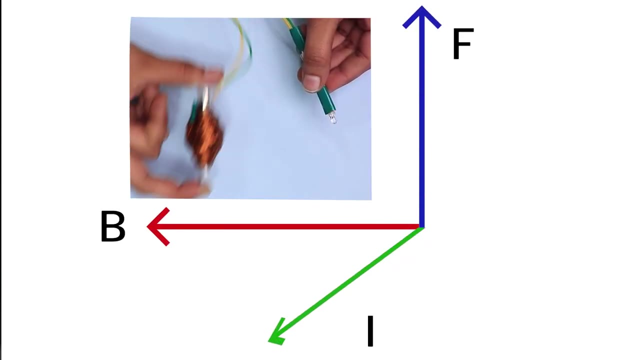 perpendicular to each other, then fleming's right hand rule states that the middle finger denotes the direction of the current, the forefinger denotes the direction of the magnetic field and the thumb denotes the direction of motion of the conductor. again, you can encourage students to find out these directions. 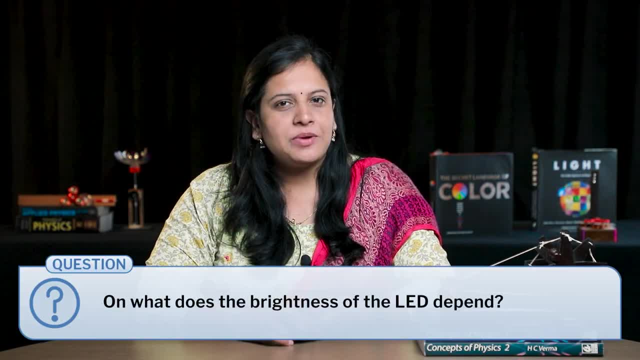 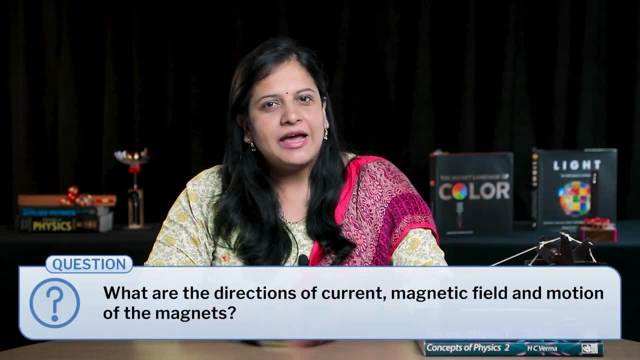 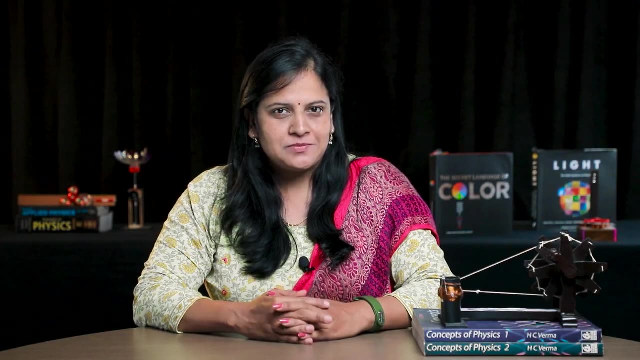 we can also ask the following questions: on what does the brightness of the led depend? you can also ask that: what are the directions of current magnetic field and motion of the magnets? now, with this, let's see how it works. Let's see one more interesting activity on the concept of electromagnetism. 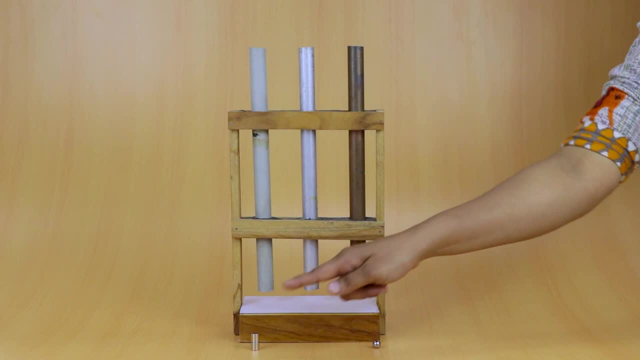 For this activity we will need a neodymium magnet, a piece of iron or steel, a PVC pipe, an aluminium pipe, a copper pipe and a stopwatch. Take a neodymium magnet and a piece of iron or steel. Drop the piece of iron or steel through each pipe separately and observe the time required. 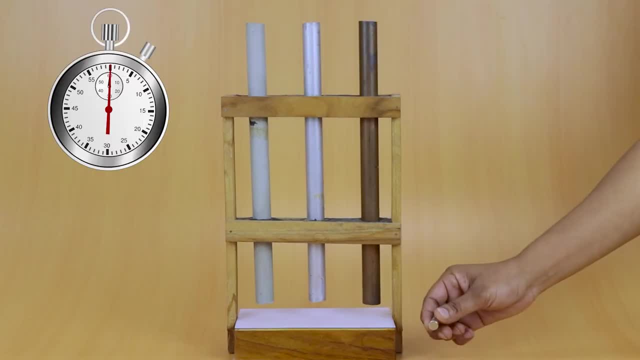 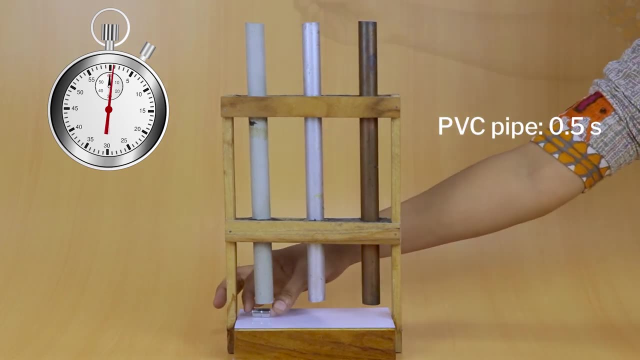 in each case. First drop the magnet through the PVC pipe and record the time taken by the magnet to fall. Next, drop the magnet through the aluminium pipe. This seems to be taking longer from that of the PVC pipe, doesn't it? 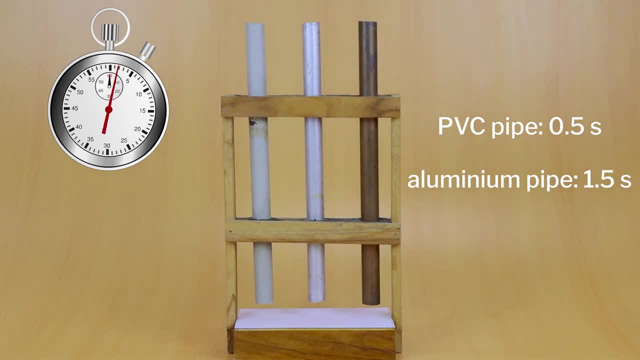 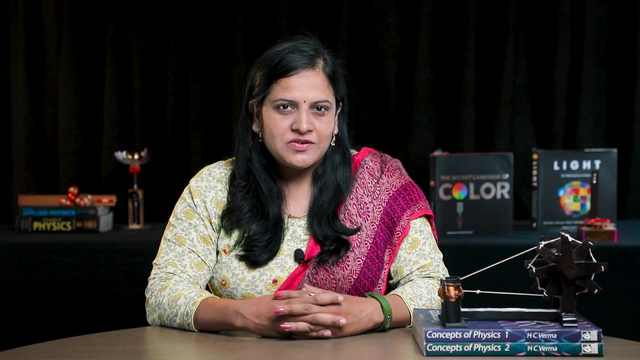 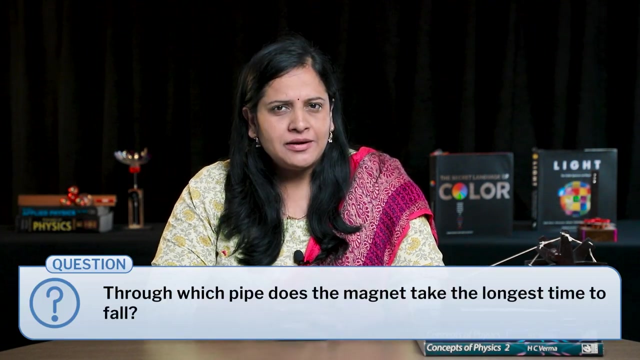 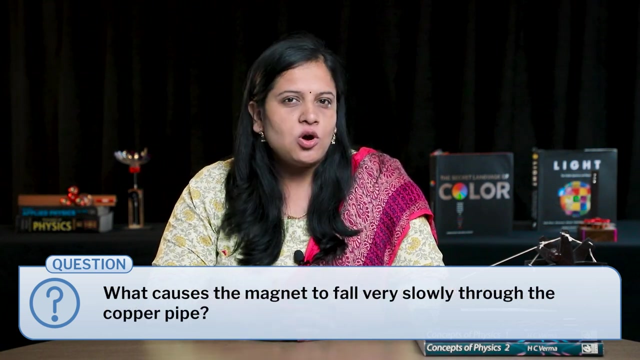 Now drop the magnet through the copper pipe. This is taking even longer time. right Here you can ask students to take the observations. You can also ask them the following questions: Through which pipe the magnet takes longest time to fall? What causes the magnet to fall very slowly through the copper pipe? 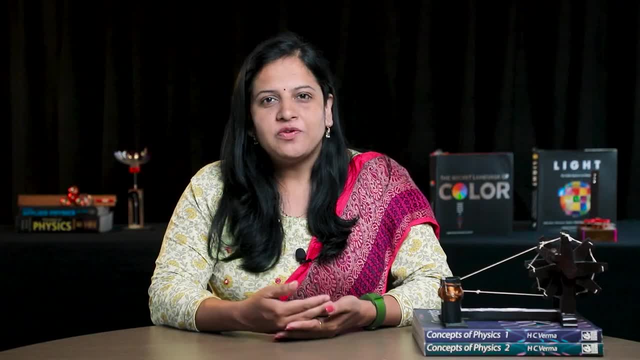 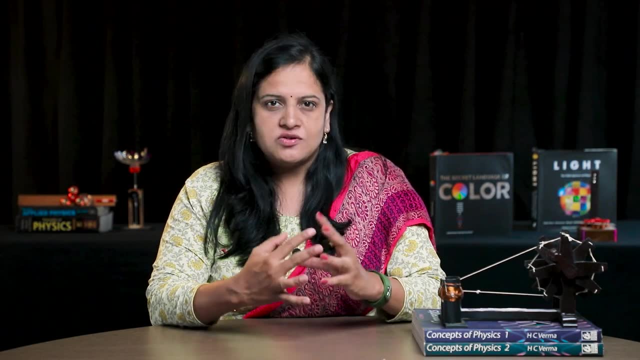 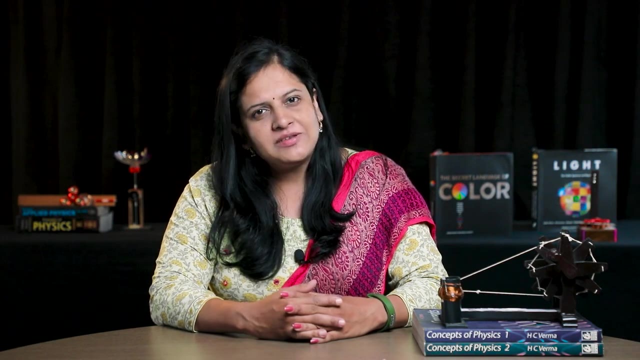 Here current follows a circular path similar to that of an eddy or a whirlpool. Copper is the best conductor of electricity amongst the three, So more current is generated. That means a more upward force is created according to Fleming's left-hand rule. 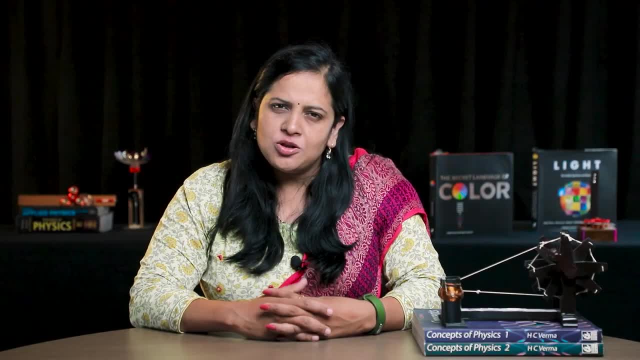 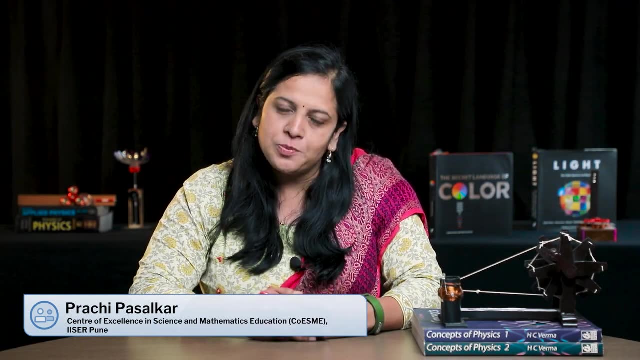 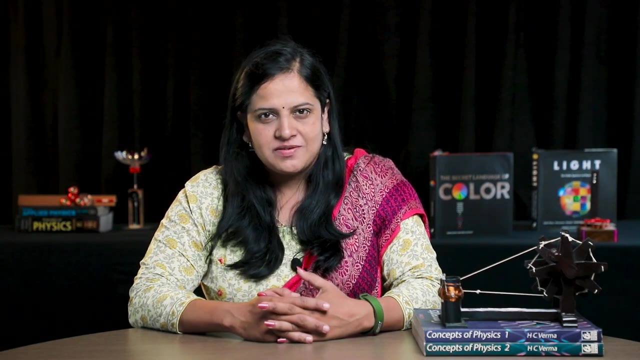 The magnet descends slowly through the copper pipe. Although we are demonstrating eddy currents, this demonstration will also help us assess students' understanding about the previous three activities. We have used materials that is cost-effective and can be reused for years. The biggest advantage of these activities is it makes the lesson more lively. 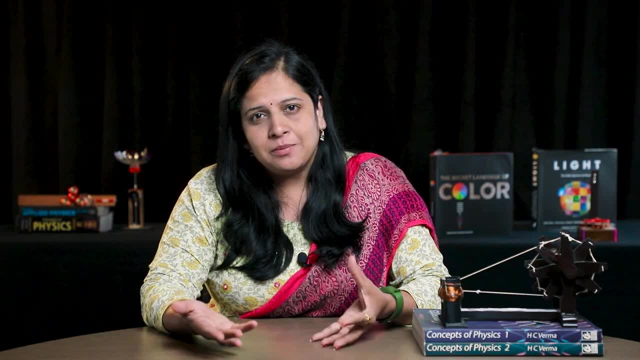 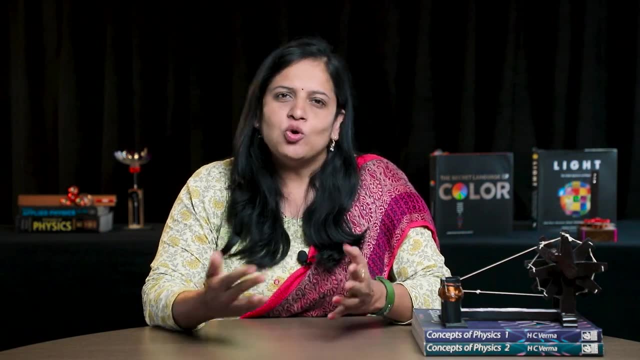 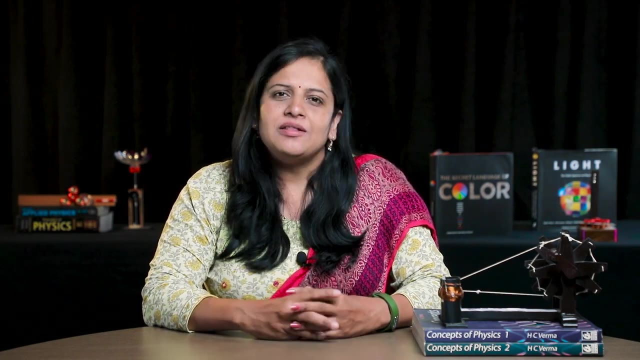 Instead of dumping definitions, equations and diagrams on students, you can use these activities, which will help them retain the concepts better. Hope this will help you, making your teaching interesting. There are more interesting activities related to this topic. Their link is given in the description box. 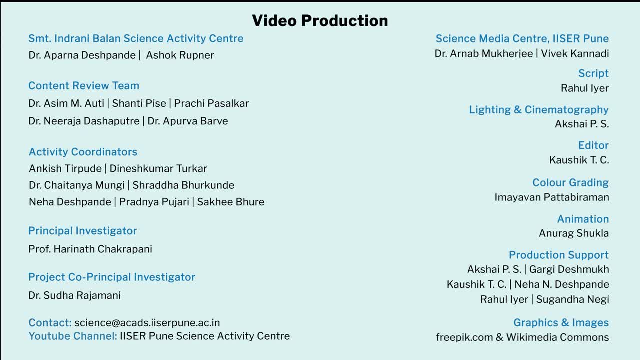 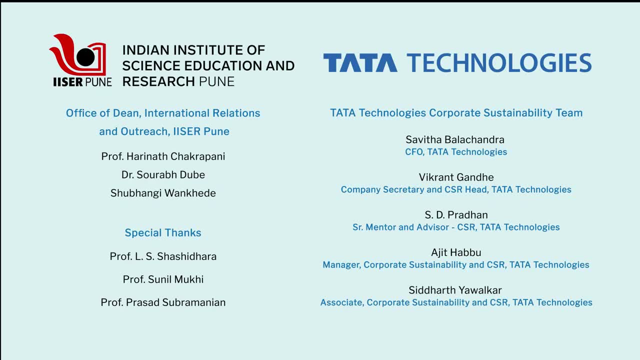 Thanks for watching. Subtitles by the Amaraorg community.